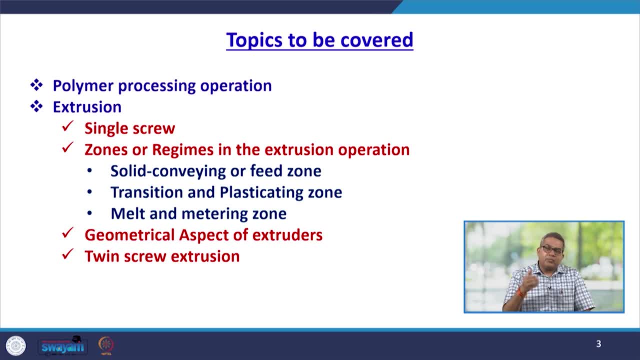 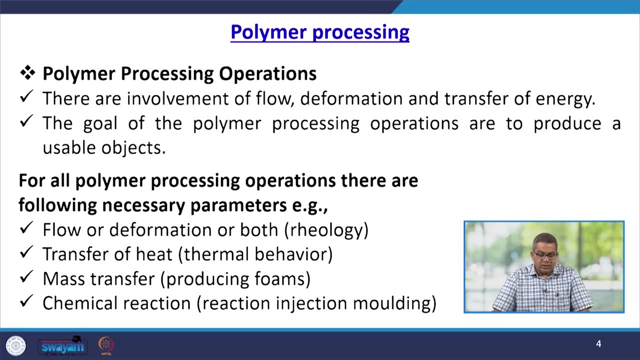 it is quite essential to have a look about this one, because it also plays a vital role in deciding the fate of a product. After this, we will have a discussion about the twin screw extrusion. Now, in the polymer processing operation, there are involvement of a flow, deformation and the transfer of 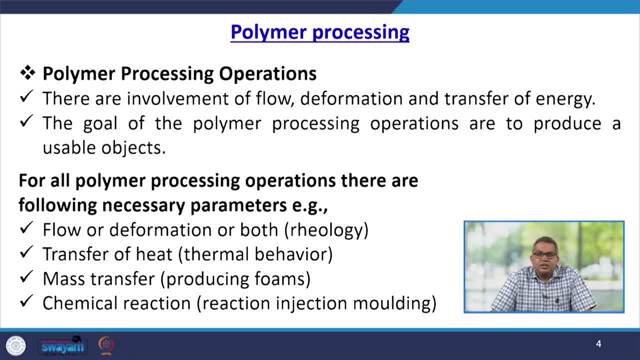 energy. The goal of polymer processing operation are: produce a usable object, a useful product. It may be commodity plastic, it may be the engineered plastic, it may be highly specialised parts. So for all polymer processing operation, various necessary parameters like flow or 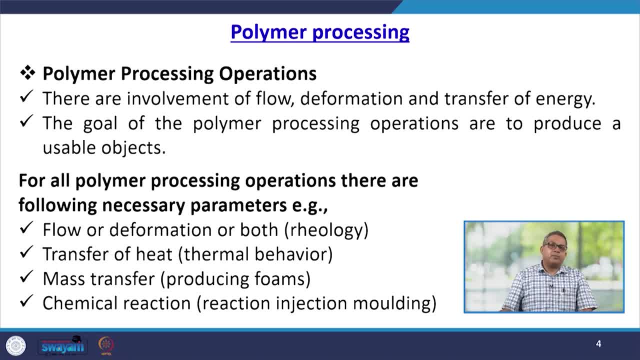 deformation or both. that means you must have a knowledge about the rheology aspect. Then the transfer of heat. that means you need to be acquainted with the thermal behaviour, how this polymer behaves when you apply the heat or when you apply the cooling. then is 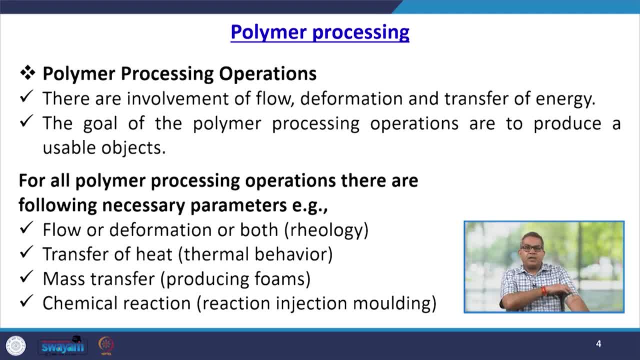 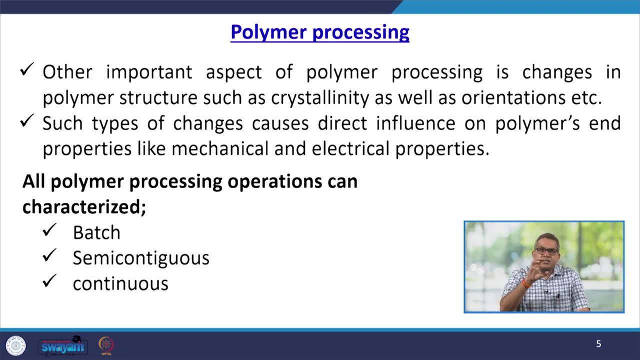 there any deformation? So all these things you need to address. Then the mass transfer. basically it is useful for producing the foams. Then the chemical reaction, that is especially the reaction injection moulding. The other important aspect of polymer processing is changes in the polymer structure, such as crystallinity, as well as the orientation. 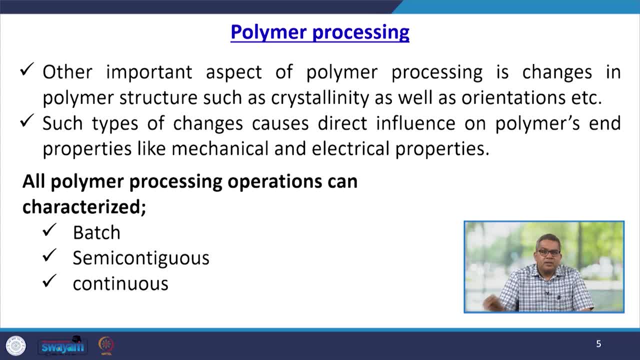 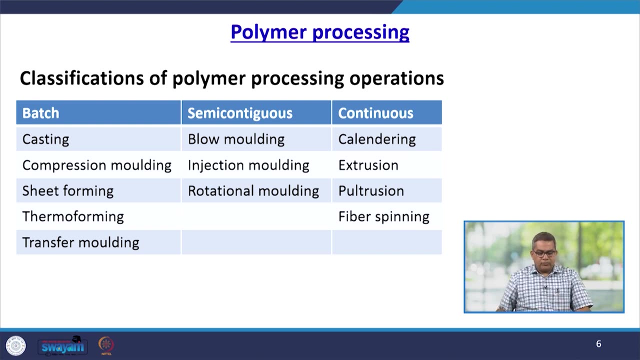 We have discussion about this one in the previous segment. Such type of changes causes direct influence on polymers and properties like mechanical and electrical properties. So all polymer processing operations can be characterised in three segments. One is batch, semi-continuous and the continuous one. Now here is the classification of a polymer processing, Like in batch we 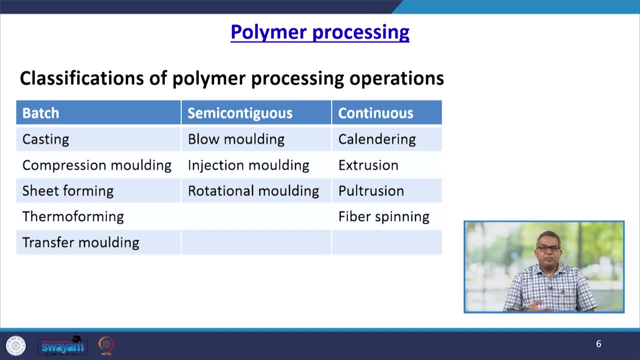 may have a casting, we may have a compression moulding, we may have a sheet forming, thermoforming, transfer moulding. all these things we are going to discuss In the semi-continuous mode. we have blow moulding, the injection moulding, the transfer moulding, the transfer moulding. 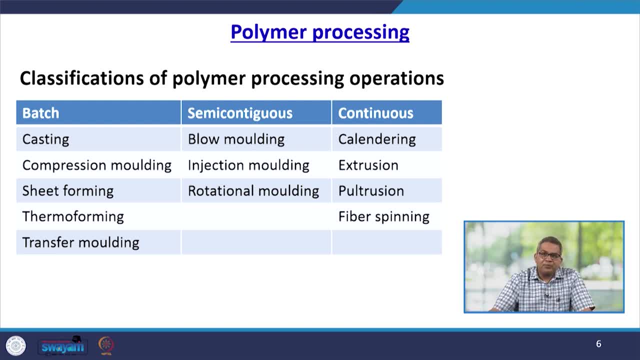 the injection moulding or the rotational mouldings, then continuous. This is the calendering: extrusion, pultrusion, fibre, spinning, all these things. So these are the various polymer processing operations. So for ease of his study, we divided all these. 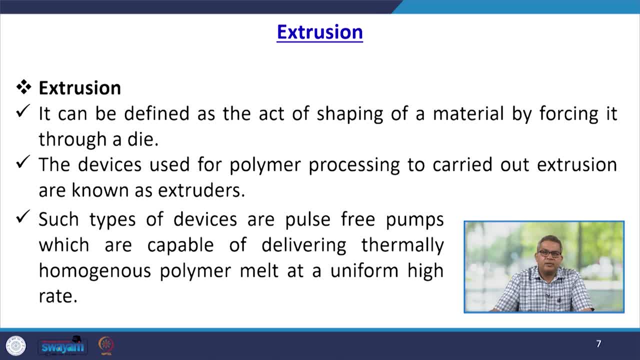 things into three segments: batch while semi continuous, and continuous. So let us start with extrusion. This can be defined as the act of shaping of a material by forcing it through your 그러면 near by the net. fearful tenía component for refused scour PE quem patient a partiàngành ep 30e in arrondiment Since the decretor or Bee. 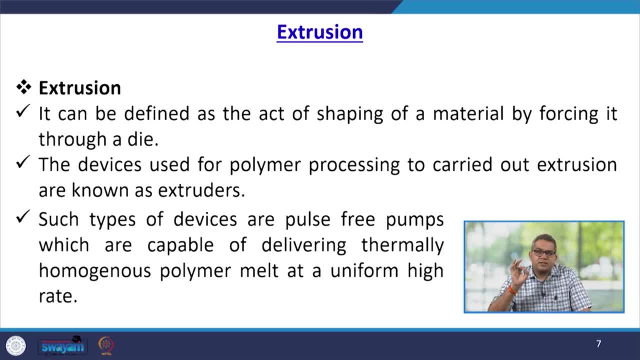 through a die. So the devices used for the polymer processing to carry out extrusion, they are known as extruder. So extrusion is a process and extruder is the machine. Now such type of devices are pulse free pumps which are capable of delivering thermally. 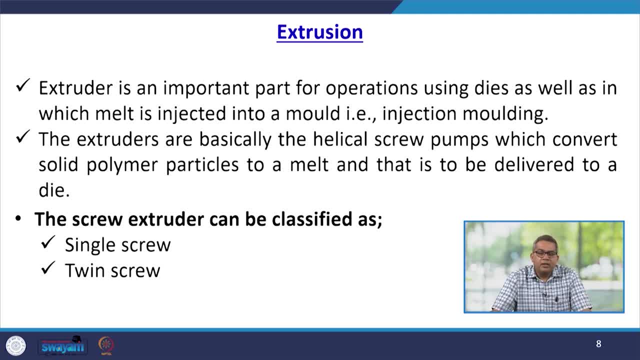 homogeneous polymer melt at a uniform high rate. Now extruder is an important part of for operation using dies as well as in which a melt is injected into a mold, like injection molding. Now the extruder are basically the helical screw pumps, which converts the solid. 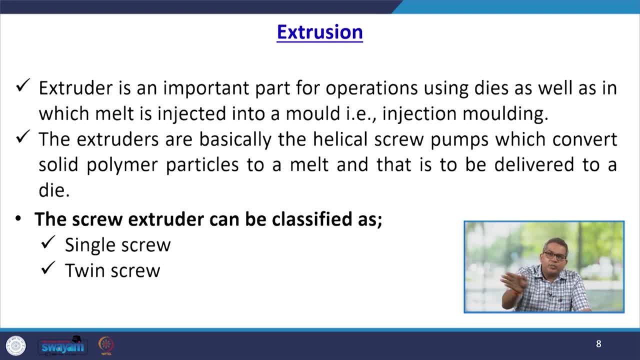 polymer particle into a melt and that is to be delivered to a die. So first thing the conversion to a melt and then it is forcefully delivered to a particular die. So the screw extruder- because extruder is the main component, this can be classified as a single screw and a twin screw. 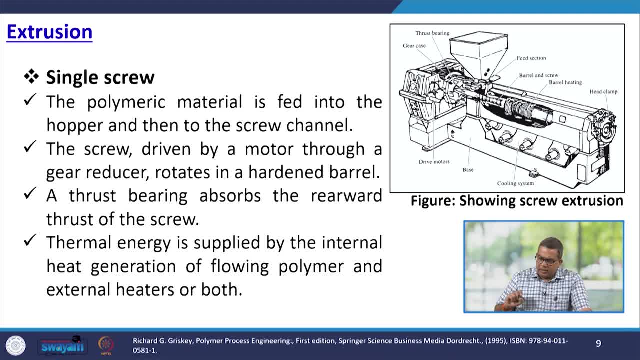 Now let us talk about the single screw. This is the typical. you see the screw extrusion, The polymeric material, as usual, is fed into the hopper here and to the screw channel, like this. Now the screw is usually driven by a motor through a gear reducer, rotates and harden. 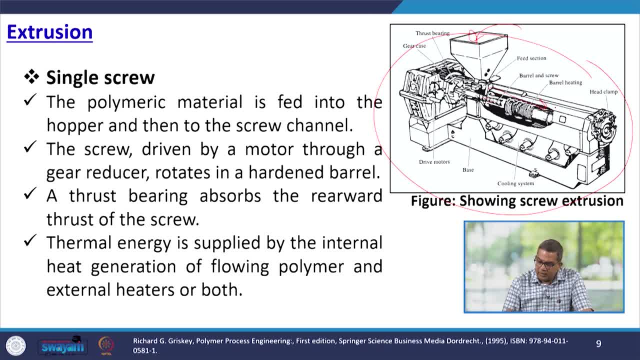 the barrel. Now, this is the barrel and this is the barrel heating zone and this is the feeding section. and you see, this is the gear case and this is the drive motor which runs the things, and here you may have a cooling section, the base. 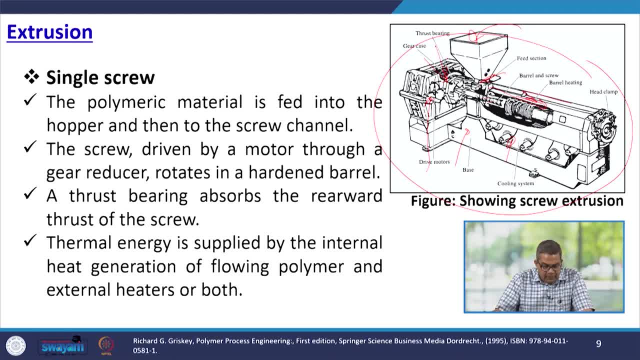 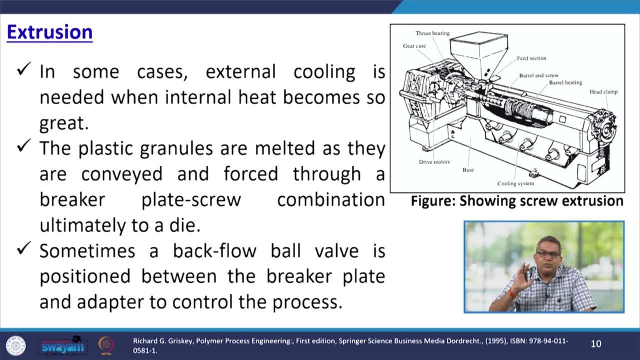 Now a thrust bearing. this is the thrust bearing absorbs and rewards the thrust to the screw. The thermal energy is supplied by the internal heating, Heat generation, like here, of flowing polymers, and external heaters, or sometimes both. In some cases, the external cooling is also needed when internal heat becomes so great. 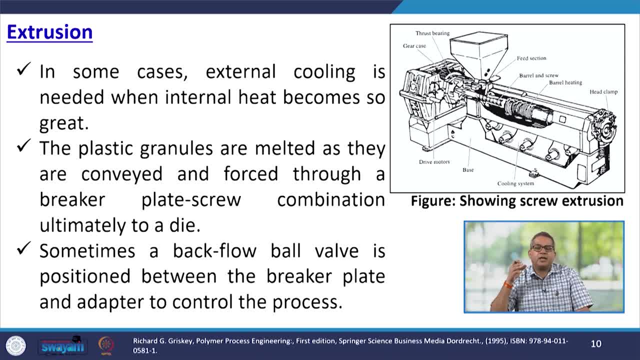 because, you see, the frictional heat is again a very crucial. It also add to the material. So whenever the heat goes up then you need to have some external cooling. So that is why there is a cooling system. The plastic granules are melted as they conveyed and forced through a breaker and a plate screw. 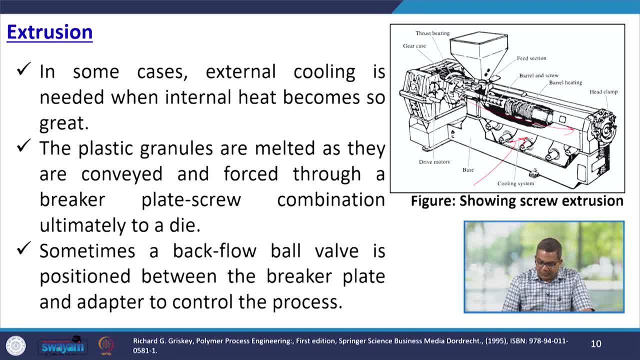 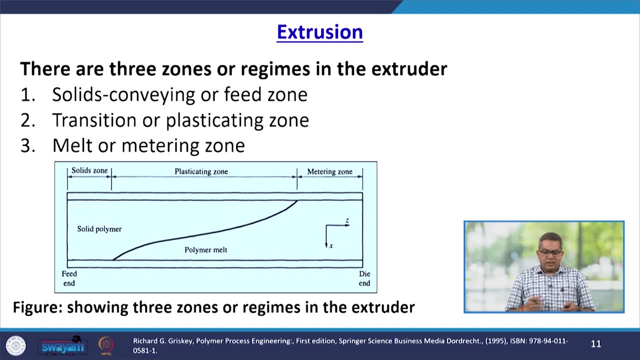 combination, ultimately to a die. Sometimes a backflow valve is positioned between the breaker plates and the adapter to control the process. Now there are three zones or regimes in the extruder. One is the solid conveying or feed zone, Then second is the transition or plasticating zone, and third one is melt or metering zone. 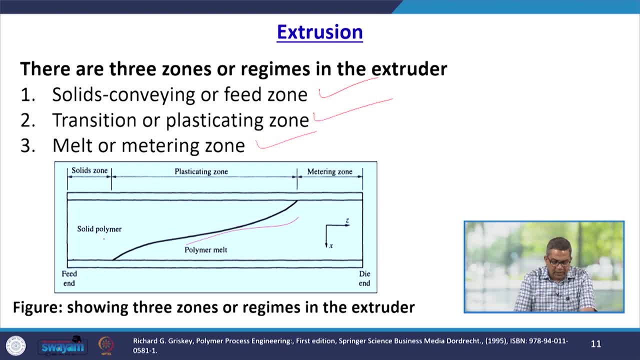 So if we plot, then you see that this is the melt and a solid polymer. This is the solid zone, This is the plasticizing zone, Then this is the metering zone and here you see that this is a die end. Now, solid conveying or feed zone. 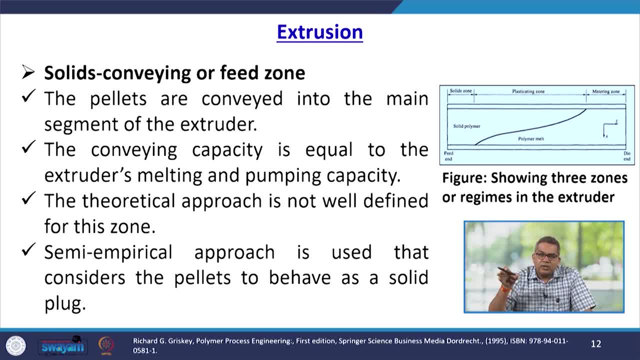 The pallets. they are conveyed into the main segment of the extruder. if you recall, the figure of the extruder and the conveying capacity is equal to the extruder's melting and pumping capacity. So the theoretical approach is not well defined for this particular zone. 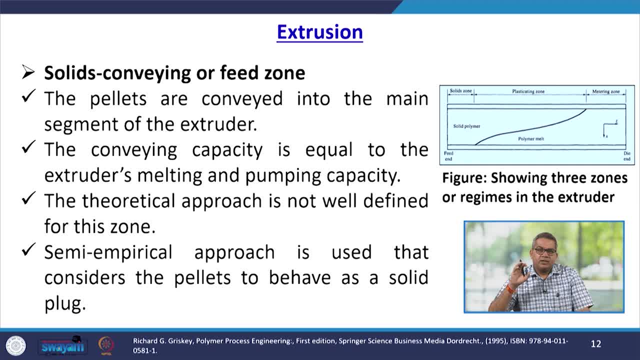 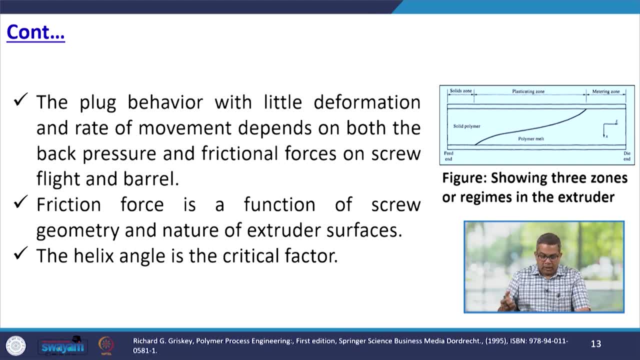 Now the semi-empirical approach is used that considers the pallet to behave as a solid plug. Now the plug behaviour. 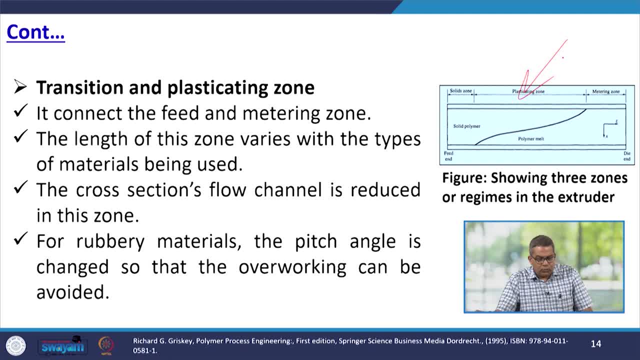 Now let us talk about the plasticating zone, or a transition zone. It connects the feed, This is the feed and this is the metering zone. It connects the feed and metering zone. The length of this zone varies with type of material being used. 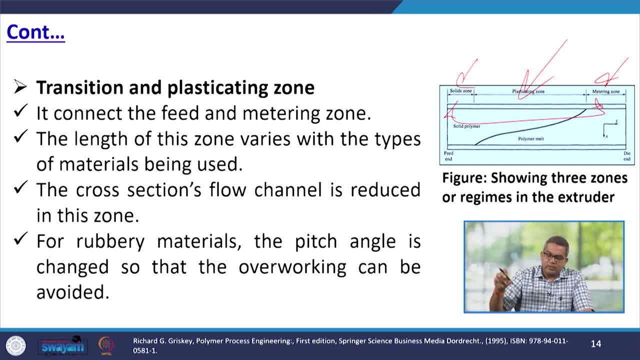 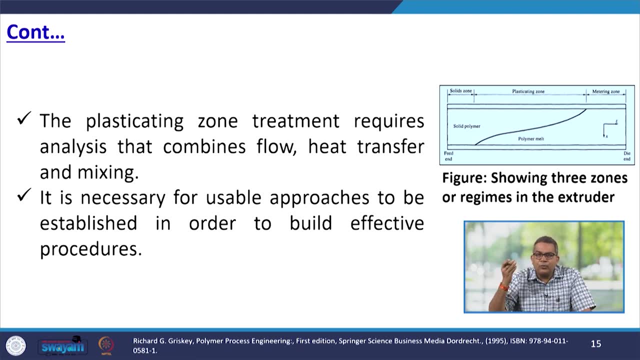 The cross section of flow channel is reduced in this particular zone. so, like this, For the rubbery material, the pitch angle is changed so that the overworking can be avoided. For the plasticating zone treatment, this requires the analysis that combines the flow. 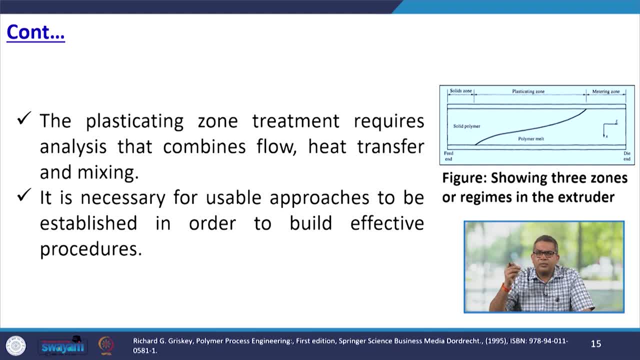 the heat transfer and the mixing. Mixing is again very important because the granules are there. sometimes you need to add some dyes and other things. So the mixing and heat transfer, because your heating, as well as the frictional heat, is also being generated, so you need to augment all those heat and you need to maintain a 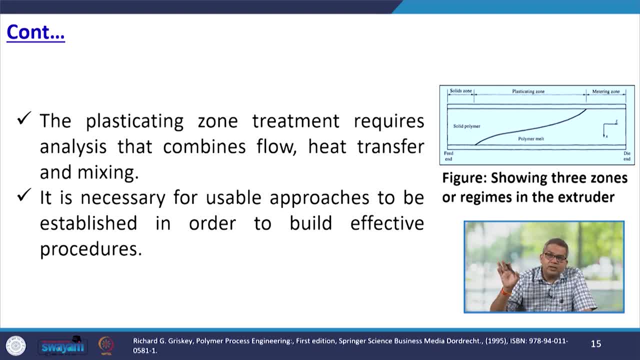 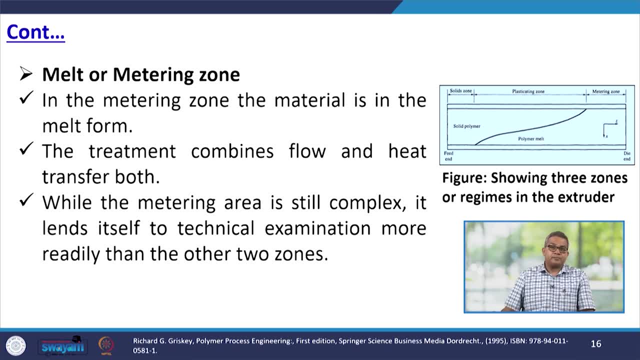 proper temperature. Now it is necessary for usable approach to be established in order to build the effective procedures. That means the optimisation is quite essential. Let us talk about the melt or metering zone. In the metering zone, the material is in the melt form. 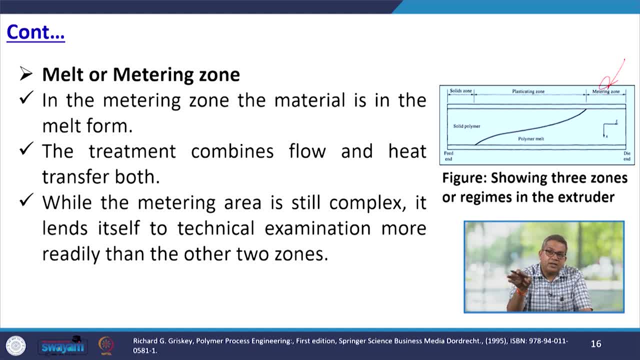 That is why the glass transition temperature and a melting temperature- the knowledge about these two temperature- is quite essential. The treatment combines flow and heat transfer, both Now, while the metering area is still complex, It lends itself in the technical examination more readily than other two zones. 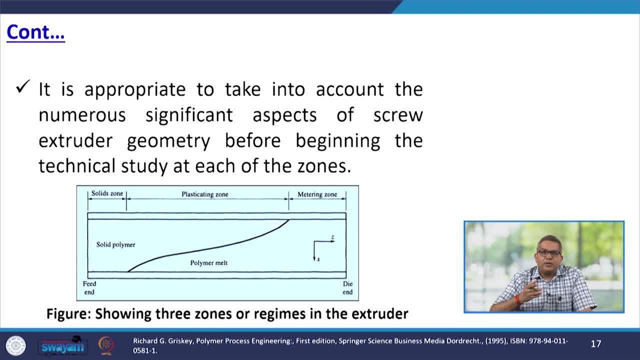 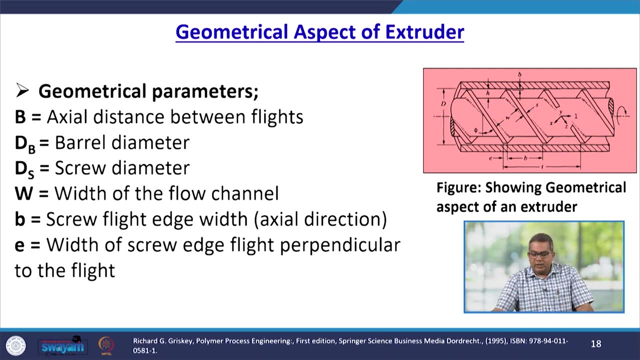 Now it is appropriate to take into account the numerous significant aspect of screw extruder geometry before beginning the technical study at each of the zone. Now let us discuss about the geometrical aspect of the extruder. Now, here, before we start, 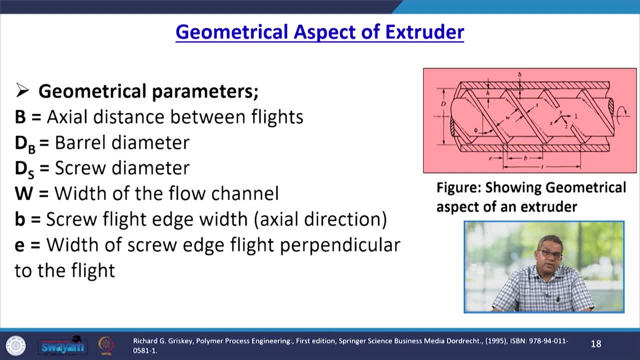 1. Toksir, To discuss about the various geometrical parameters. this geometry plays a very vital role not only towards the mixing but also for the heat segment and the further movement of the polymeric material. So there are various geometrical parameters associated in this particular study. 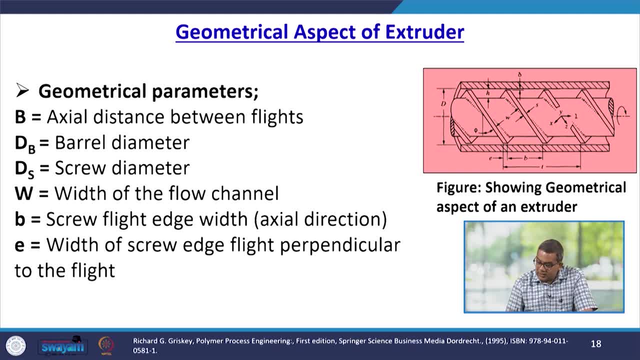 One is the axial distance between the flights like this: these are the flights, So you need to know about the axial distance between the flights. Then you must know about the barrel diameter: what is the diameter of the barrel? Then screw diameter: what is the screw diameter you need to know? and that is referred as ds. 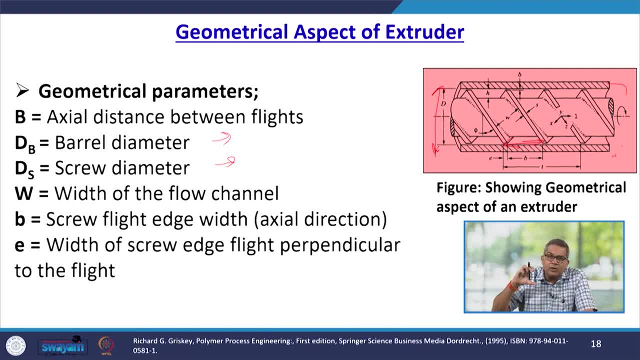 and db in the usual notations. Then w, that is the width of the flow channel. you must aware about this w aspect. Then screw flight, Then edge, with the axial direction and width of screw edge flight perpendicular to the flight. So all these parameters you must know. 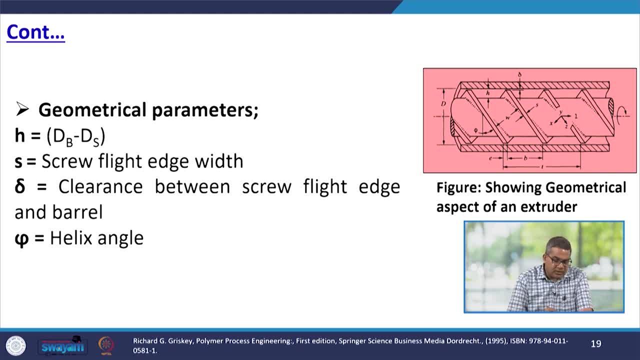 Apart from this, you should know about, say h, that is, the barrel diameter and screw diameter, the difference between the barrel diameter and screw diameter, Then screw flight edge width, that is referred as s. Then this is again a very important and you should know about this one before deciding. 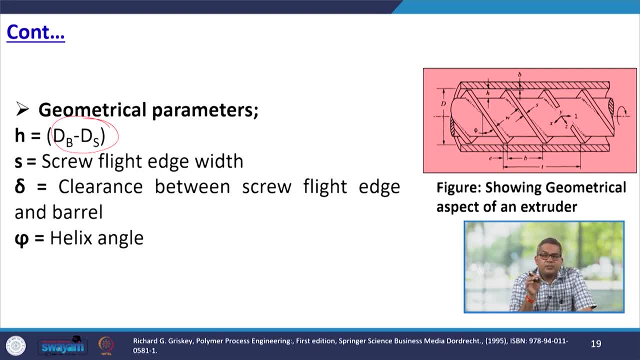 Then clearance between the screw flight edge and the barrel. this should be needed because this is essential for the free movement of the polymer towards the forward direction. So this is referred as the delta, Then helix angle, that is psi. This is the helix angle. 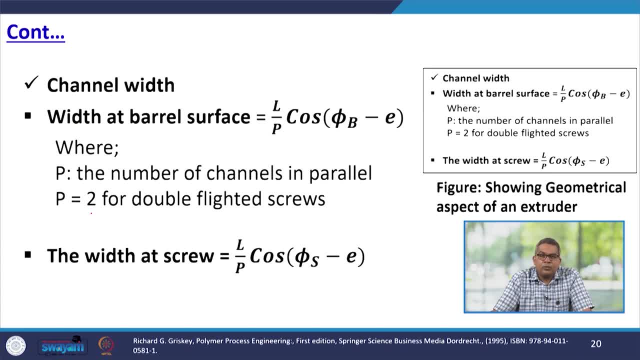 So this is again very important to know: The channel width. The channel width, The channel width- Usually this is width at a parallel surface and referred as L by P, cos, phi, b minus e, where P is the number of channels in parallel and P is equal to 2 for double flight screw and 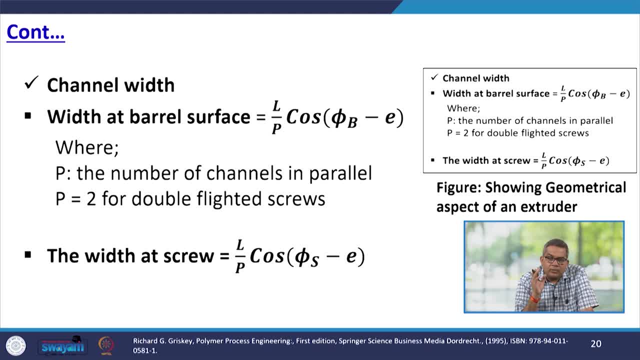 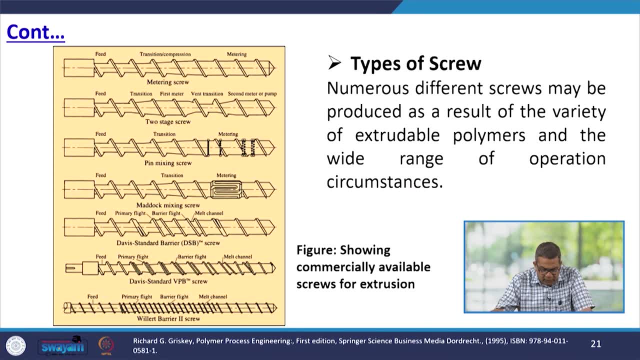 the width screw is L by P cos phi s minus e. This reflects the geometrical aspect of this extruder. Now here The new architecture, The numerous different screws. they may be produced as a result of a variety of extrudable polymers and a wide range of operation circumstances. 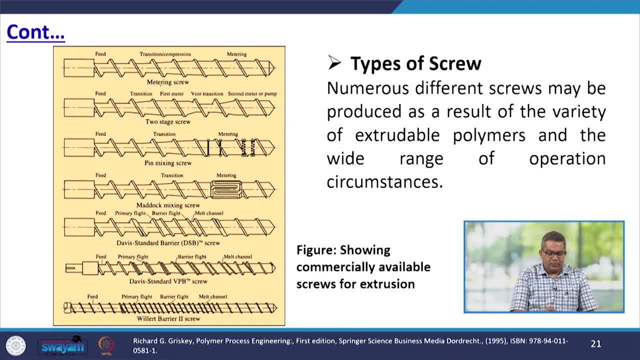 Here you see that the commercially available screws like. you see that metering screw, two stage screw. pin mixing screw. you see the difference in the shape. Then Maddock mixing screw. Davis standard barrier screw. Davis standard screw. Willard barrier screw. 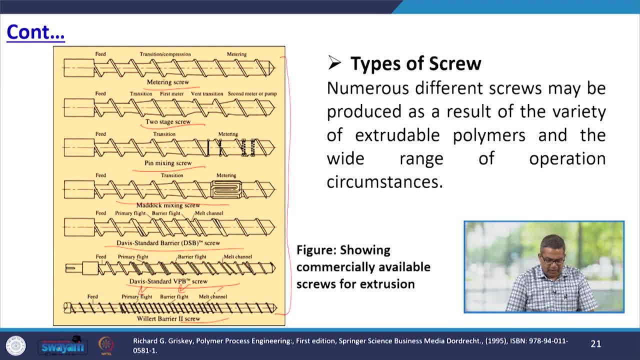 All these things, you see that different. the prime flight barrier, flight melt channel. so all these are difference. you can easily analyze that there is a difference and this all depends on the processing condition. it all depends on the polymers being used for the process in question. 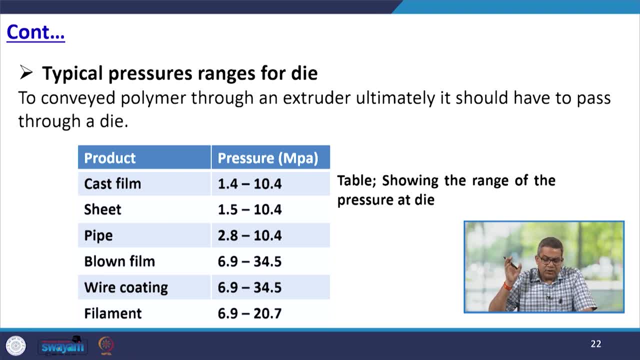 Now there is again crucial aspect is that typical pressure ranges for the die, because ultimately the melted polymer will flow through die. Now to convey the polymer through an extruder, ultimately it should have to pass through a die. So usually there are different type of a product and enlisted the pressures, like cast film. 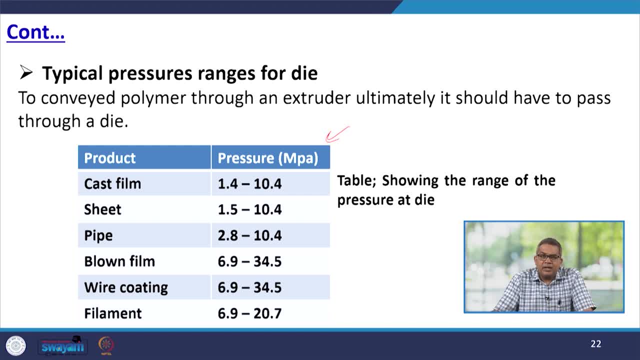 they must have 1.4 to 10.4 megapascal, then sheet 1.5 to 10.4, then a pipe. usual process for producing pipe is the extruder, So 2.8 to 10.4.. 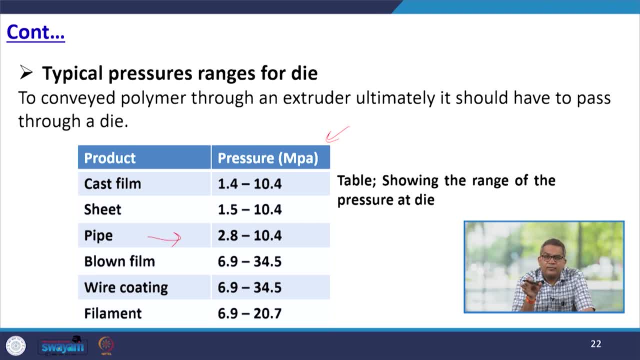 Then the blown film 6.9 to 34.5 and the wire coating 6.9 to 34.5 megapascal and the filament 6.9 to 20.7. and you see the variation and this reflects that the product how much they. 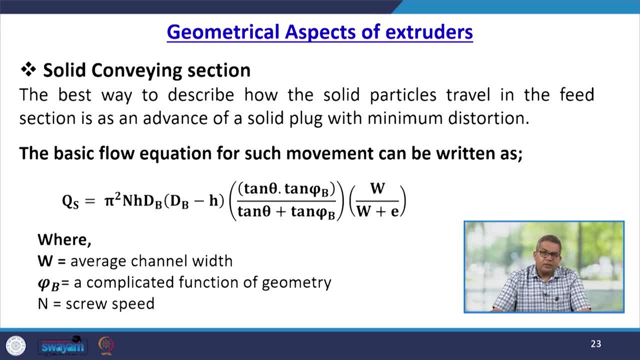 are sensitive towards the pressure. Now, another thing is that the solid conveying section- the best way is to describe how the solid particles travel in the feed section. The feed section is an advance of a solid plug with minimal distortion, So the basic flow equation of such moment can be represented mathematically like Qs is: 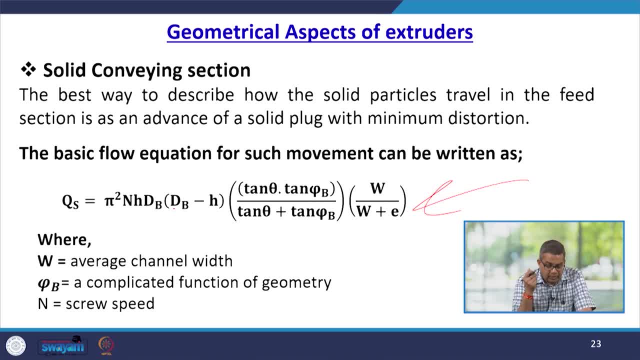 equal to pi, NH, db. db is again the barrel diameter, db minus h, tan theta minus tan psi. for the barrel, which we have already discussed over tan theta plus tan psi b, that is for the barrel, This is equal to W upon W plus E, where W is average channel width, psi b is a complicated 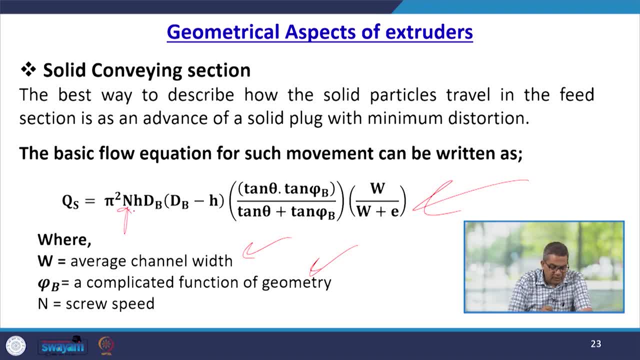 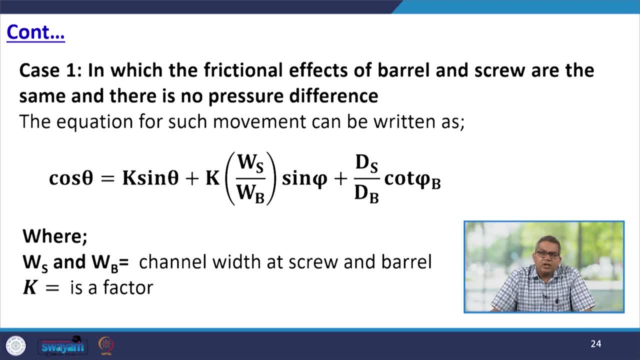 function of geometry, and this N is the screw speed. Now let us discuss couple of cases in which. in the case 1, in which the frictional effect of the barrel and the screw are the same and there is no pressure difference, So the equation for such moment can be mathematically represented as: cos. theta is equal to K sin. 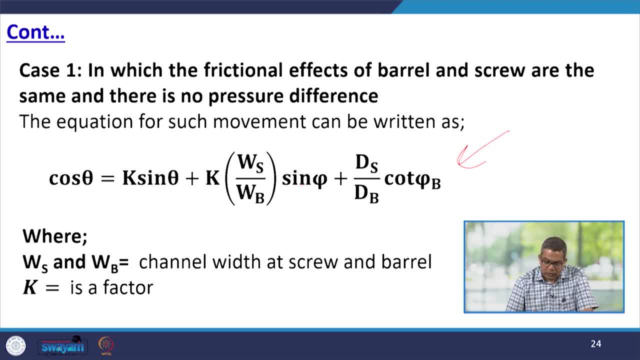 theta plus Kws over Wb. So this is the frictional effect of the barrel and the screw are the same and there is no pressure difference. Another case is the frictional aspect. So for example, let us take the yea psi dp into sin. psi plus ds over db cot psi b where 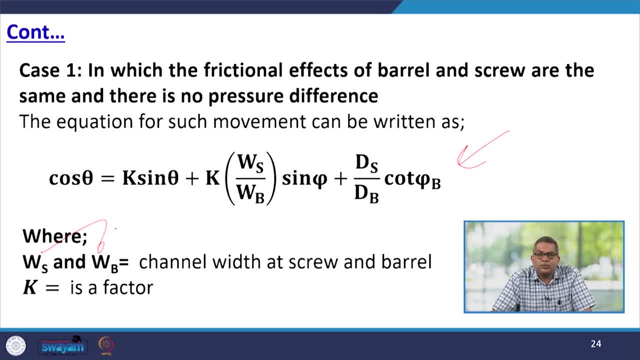 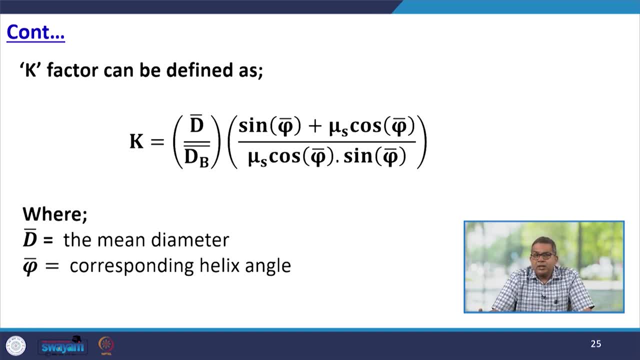 Ws and Wb. these are the channel width of the screw and barrel and K is the factor. Now the question arises that how we can determine the K factor. Now this K factor can be determined as K is equal to d over db, sin psi plus mu s cos psi. 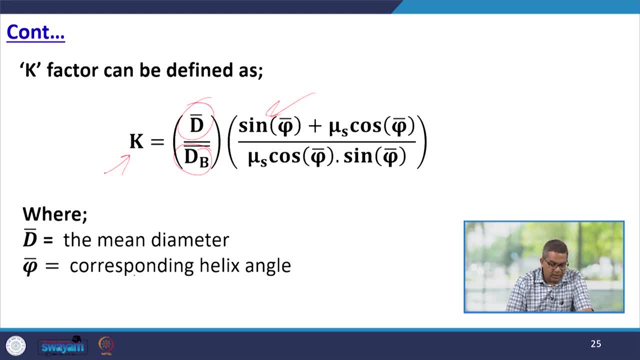 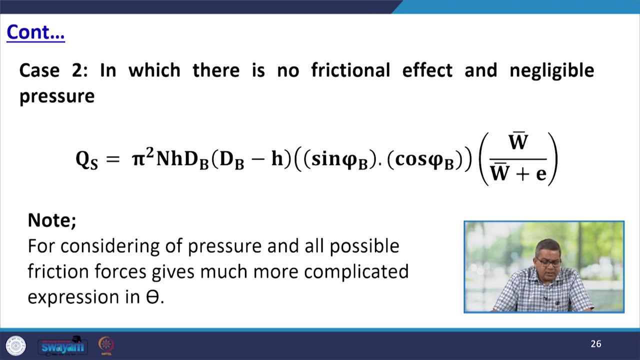 over mu s cos psi into sin psi. Okay, where D is the mean diameter and psi is the corresponding helix angle. We have already discussed the helix angle in the previous slides. Another case in which there is no frictional effect and negligible pressure. so in that 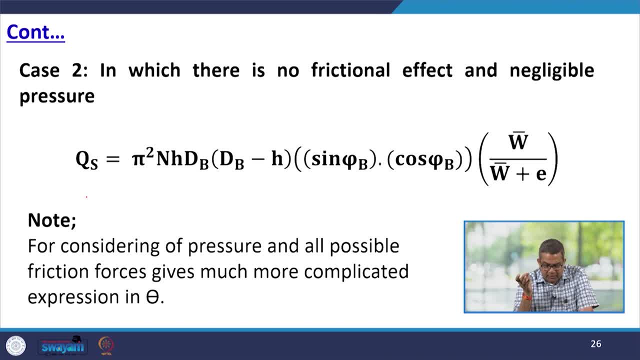 case, all the notations as per the previous discussion. now Q s is equal to pi square N, H, db. db is the barrel diameter, db minus H. then sin psi b into cos, psi b into W over W plus E. Now for considering of a pressure and all possible friction forces, given much. 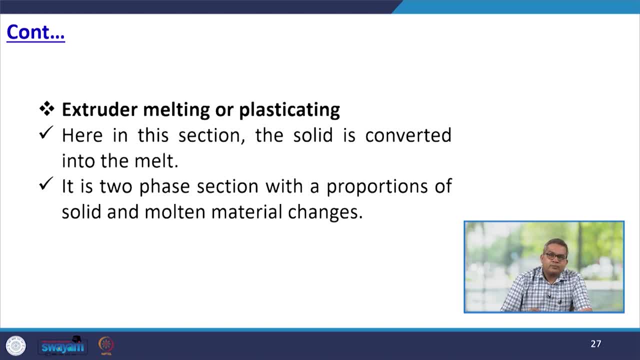 more complicated expression, N? theta, Now extruder, melting or plasticating. Now, in this particular section, the soil is not hot, only solid is converted into melt. So again, I am emphasize that the knowledge about the T? m, that is, the melting temperature and a glass transition temperature, is quite essential. 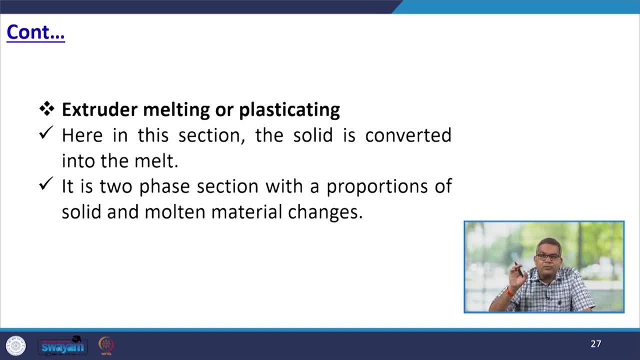 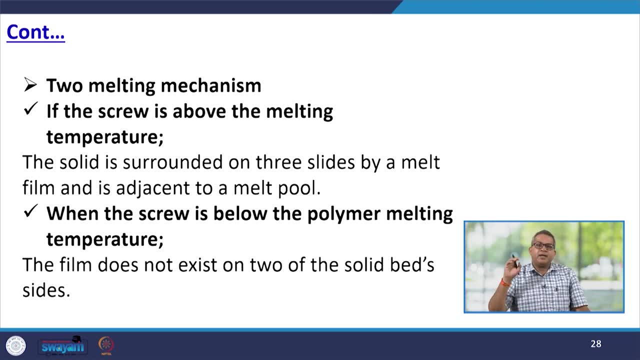 Now it is a two phase section with a proportion of solid and a molten material change. Now there are two melting mechanisms. One is that if a screw is above the melting temperature, So the solid is surrounded by a solid. So watch this. 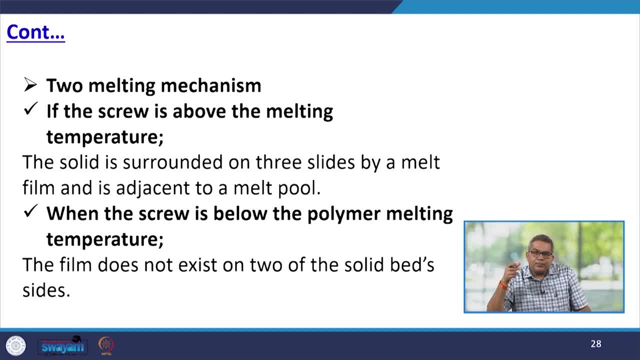 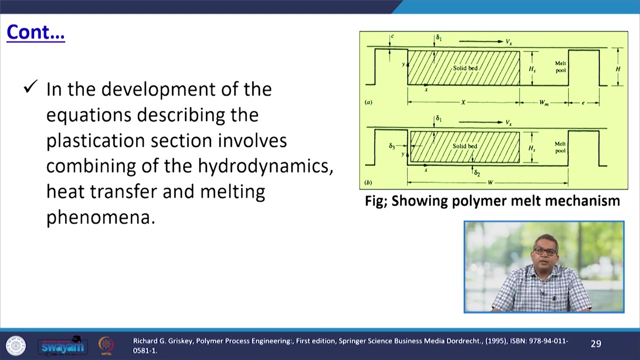 surrounded on three slides by a melt film and adjacent to a melt pool. So and second case is that when the screw is below the polymer melting temperature, so the film does not exist on two of the solid beds. slide Now in the development of the equation describing the plastication section, this involves the 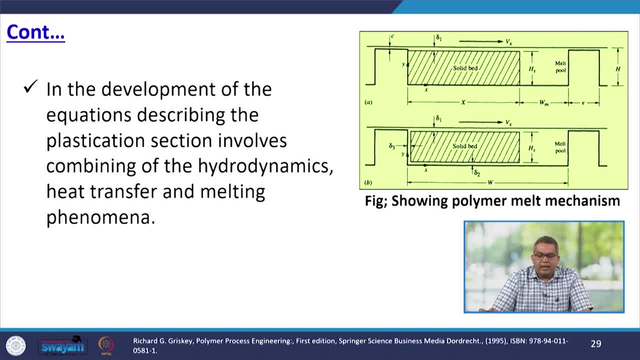 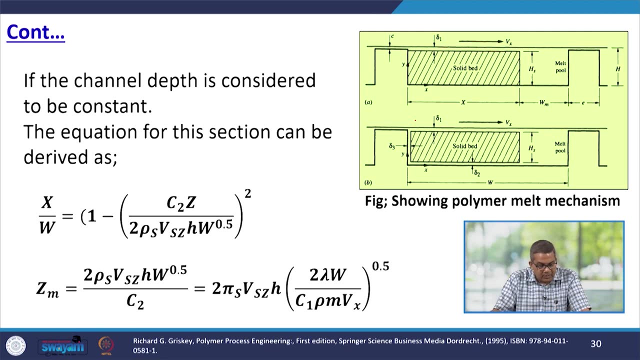 combining of hydrodynamics, heat transfer and melting phenomena. Now this: you see that this particular figure shows the polymer melt mechanism, like here, the solid bed and this is the melt pool. So different segments just need to be addressed. Now, if the channel depth is considered to be constant, obviously this is an assumption. 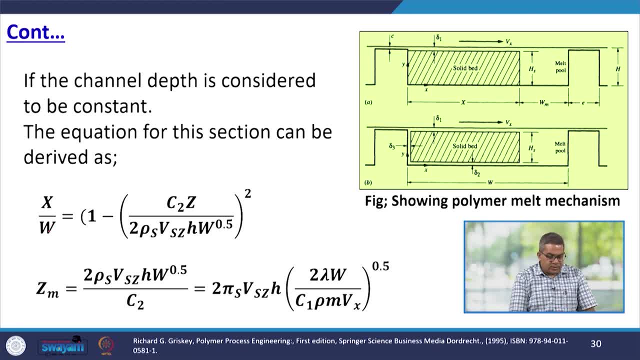 the equation for this section can be So: Z m X over W is equal to 1 minus C 2. Z over 2 rho S VSZ, H, W to the power 0.5, and this whole is square. Z m is equal to 2, rho S VSZ, H W to the power 0.5 over C 2 is. this is equal to 2 pi S VSZ. 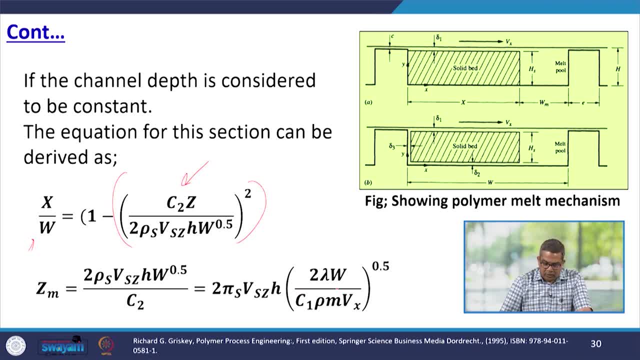 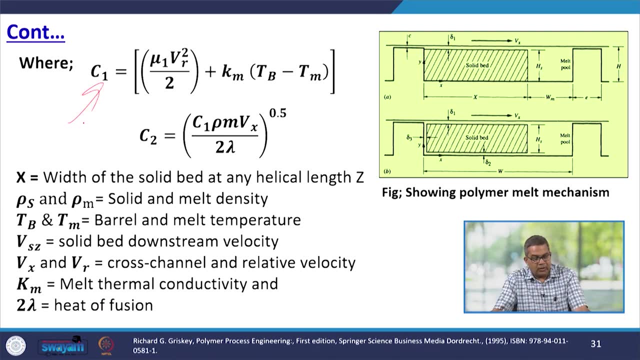 H into 2 lamda, W over C, 2 muscle, This whole square, C1, rho, m, Vx to the power 0.5.. Now here we have discussed the two terms C2 and C1.. So where C1 is equal to mu, 1 into Vr, square over 2 plus Km, into Tb minus Tm, and we are utilizing 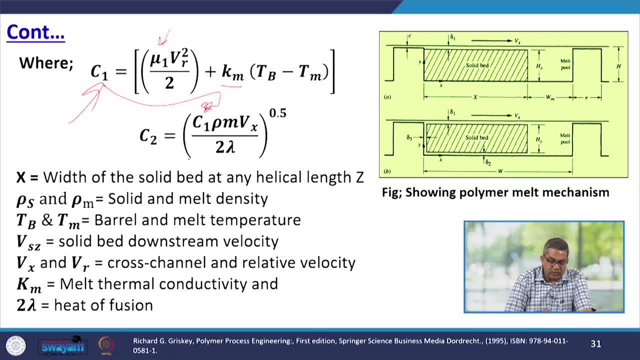 this C1 over here, that is C2. for calculation of C2, that is: C2 is equal to C1 into rho m Vx over 2 lambda to the power 0.5.. Now here x, we have utilized the x, here x, that is the. 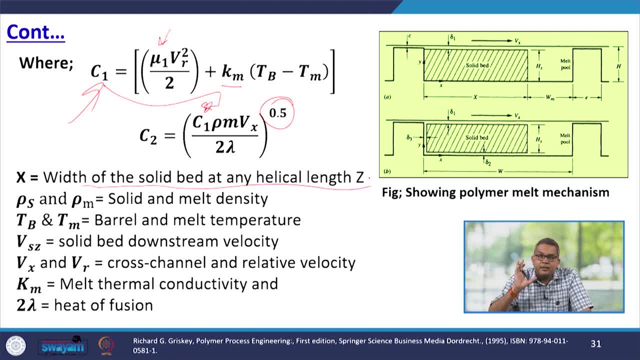 width of the solid bed at any helical length: z, Now rho s and rho m. this is the solid and melt density, So you must know about this one. Then Tb and Tm: this is the barrel and melt temperature. Vsx, Vsz is the solid bed downstream. 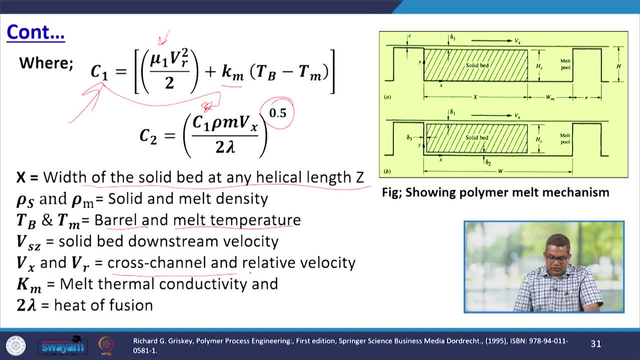 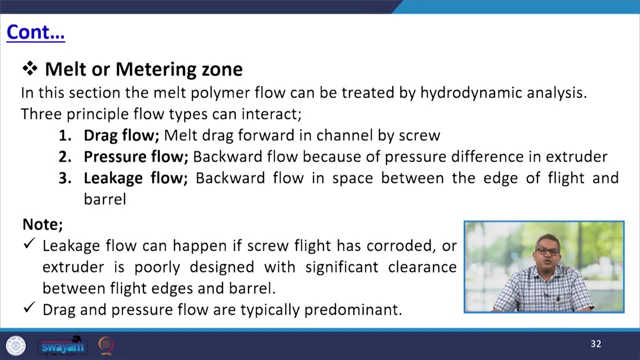 velocity, Vx and Vr- this is the cross channel, and relative velocity and Km. this is the melt, thermal conductivity and 2 lambda- that is the heat of fusion. Now let us talk about the melt or metering zone In this section, the melt polymer flow. 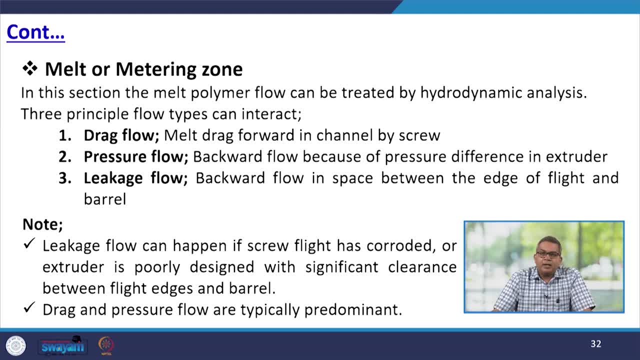 can be taken. It can be treated by the hydrodynamic analysis and usually three principle flow types which can interact. One is the drag flow, the melt drag forward in channel by screw the pressure flow. the backward because backward flow because of the pressure difference in the extruder. 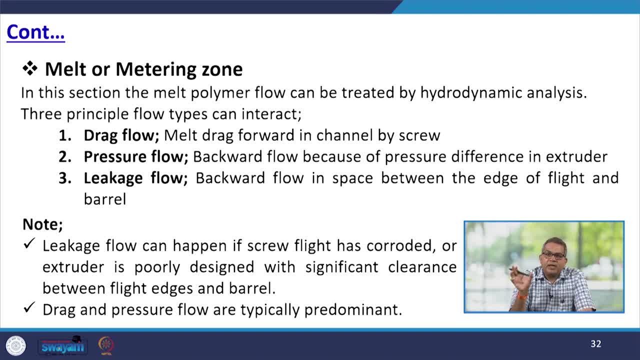 and the leakage flow, that is, the backward flow in space between the edge of the flight and the barrel, like this. So the leakage flow can happen if the screw flight is corroded or extruder is poorly designed with the significant clearance between the flight edge and barrel. Now this is the barrel. 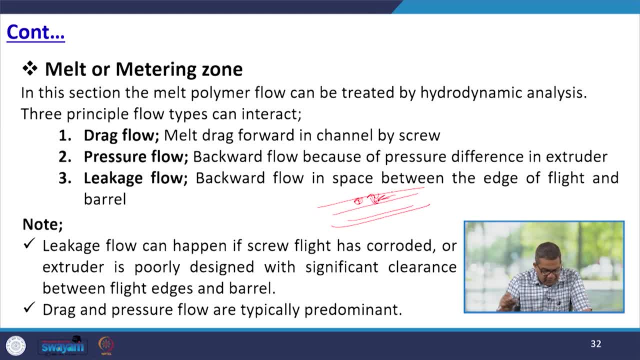 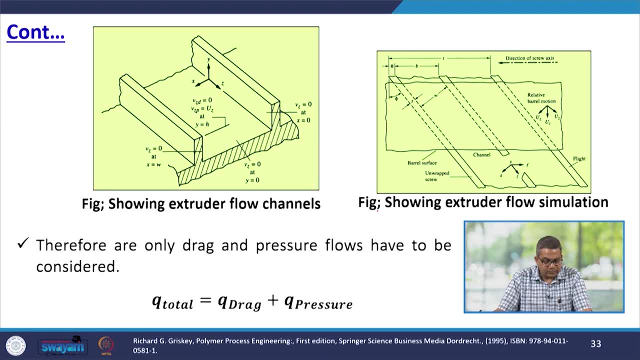 and this can create the leakage, The drag and the pressure flow. they are typically predominant Now. therefore, only drag can create the leakage. That is why we call it the roll out, roll out, and overall It is the roll out that is the drag flow, because the drag flow will take place between the 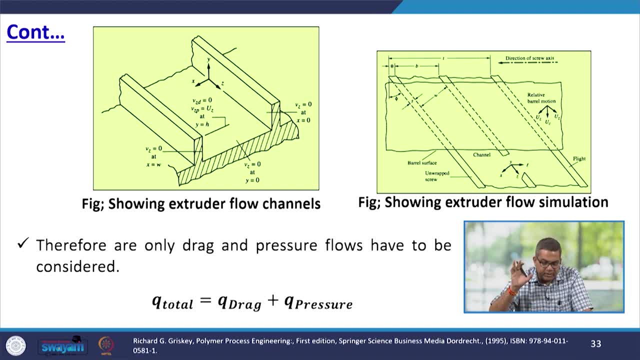 edge and barrel. The drag flow will take place between the edge and barrel If the roll out and pressure flows have to be considered. Here you see the extruder flow channels and this is the flow simulation. So when we are considering all these things, then Q total. 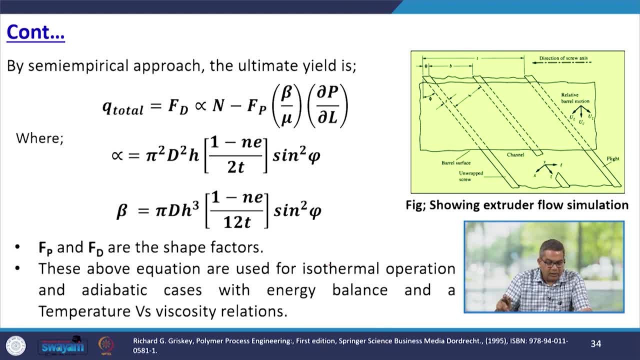 is equal to Q drag and Q pressure. So by semi-empirical approach, if we adopt the semi-empirical approach, the ultimate yield is this: is Q is a yield. So Q total is equal to FD, is proportional to N minus FP. beta over mu into del P over del L. this, sorry, this is, this one is alpha. 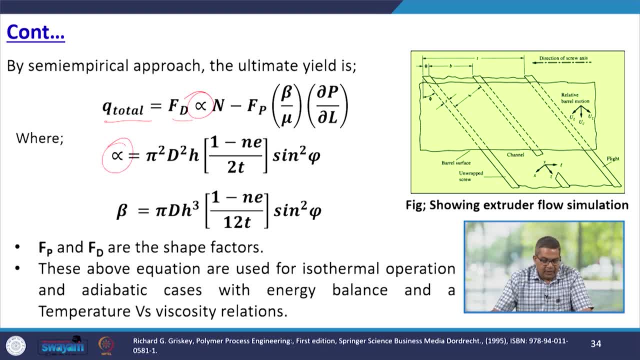 Now alpha is equal to pi square D, square H into 1 minus NE upon 2T sin square psi. So, and the beta is equal to pi DH cube into 1 minus NE upon 12T sin square, sin psi square. Now, FP and FD are the shape factors. So here this is the shape factor, Now these the above. 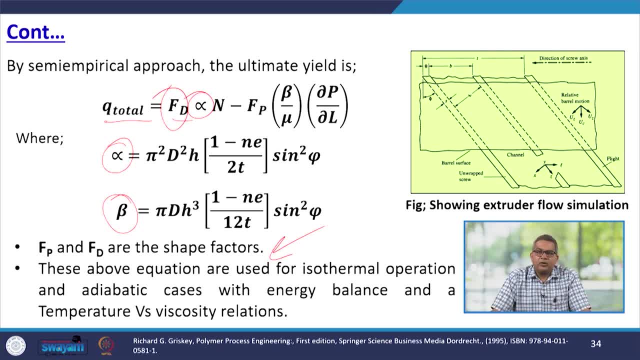 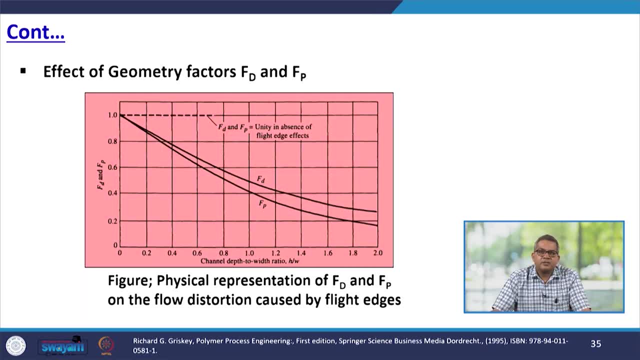 equations are used for isothermal operation and adiabatic cases, with energy balance and a temperature versus viscosity relations 3.. Now here you see that this is the physical representation of FD and FP on the flow distortion. This is caused by the flight edge. 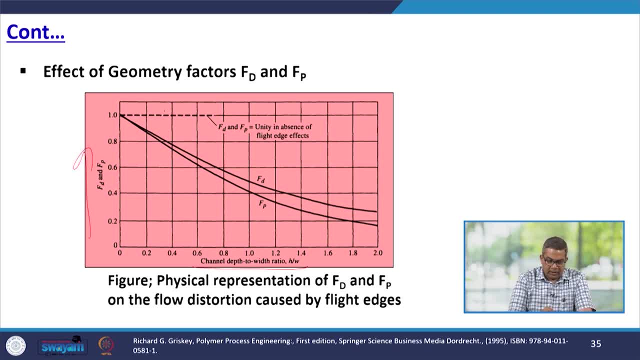 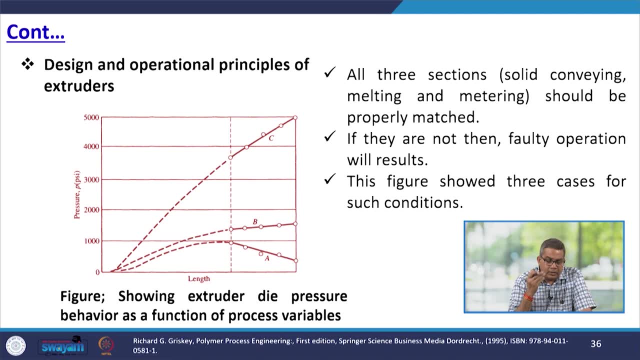 You will see the channel depth and FD and FP and you see the pattern of this one and this reflects the effect of a geometry factor: FD and FP. Now there are various principle associated with the design and operational things of extruder. So all these sections like solid conveying, melting and a metering, this should be properly. 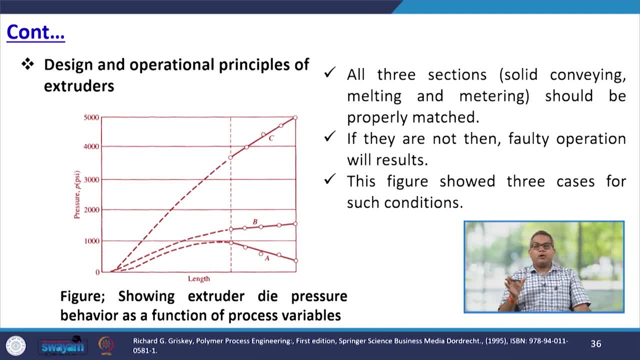 matched. There must be proper synchronization among all three sections, and if they are not, then the faulty operation may cause the deformed product. So this figure shows the three cases in such condition: length versus pressure and all these things, three sections, Solid, conveying, melting and a metering zones. they are reflected over here. 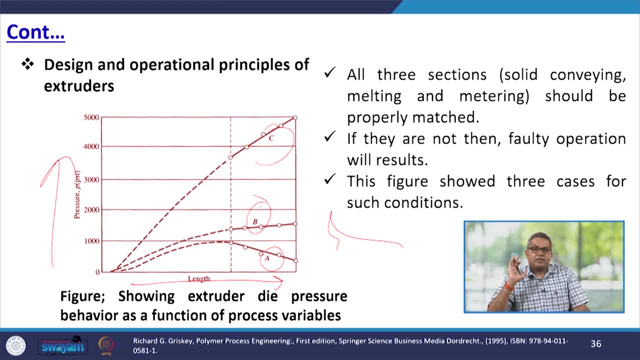 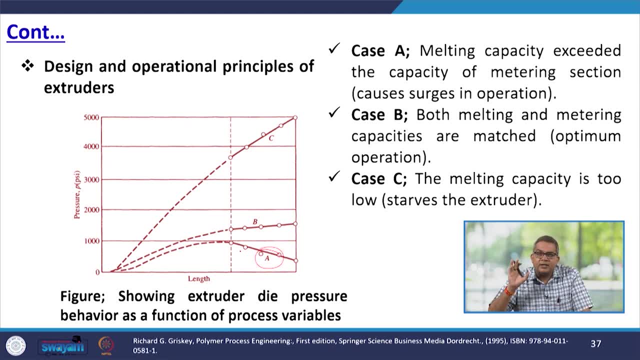 This showing the extruder die pressure behavior as a function of process variables. Now here different cases, like in case A, the melting capacity exceeded the capacity of metering section. This causes the surge in operation. Now in this case B, the both metering and melting capacities are matched. 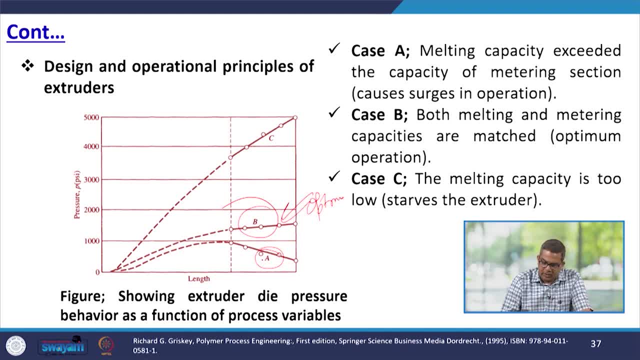 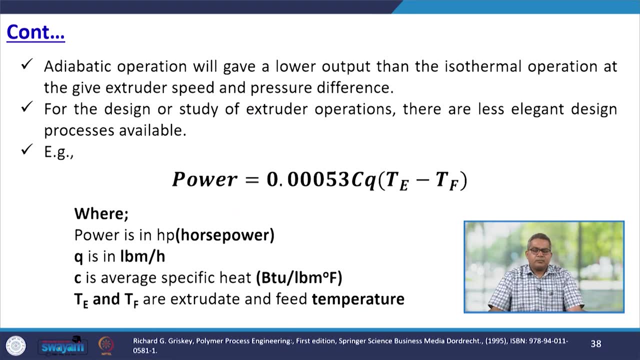 This is the optimum operation. Now here in case 3, the melting capacity is too low. This starves the extruder. So you need to have some optimum values for the smooth operation of your extruder. Now adiabatic operation. this will give a lower output than the isothermal operation and at 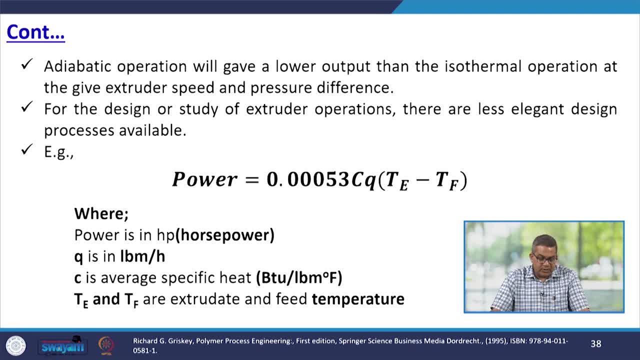 the given extruder speed and pressure difference. Now for the design or study of extruder operations. there are less elegant design processes available, like, for example: power is equal to 0.00053 CQ into TE minus TF, where power is in, usually horse power. Q is in pounds per hour, C is the average specific heat and usually represented. 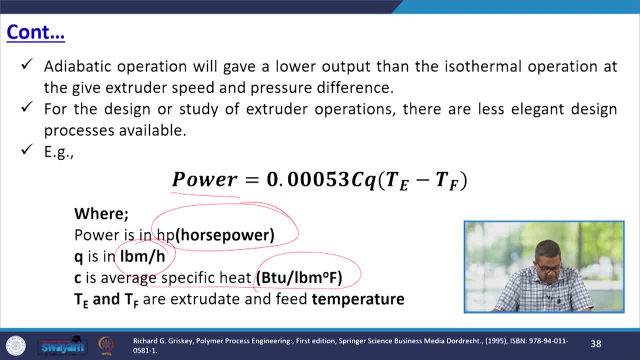 in BTU, over pounds Fahrenheit, And TE and TF are the same. So this is the average heat and usually represented in BTU, over pounds Fahrenheit, And TE and TF are the same. So this is the average heat and usually represented in BTU, over pounds Fahrenheit. 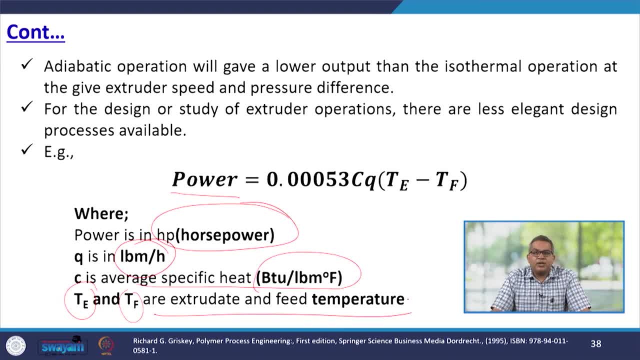 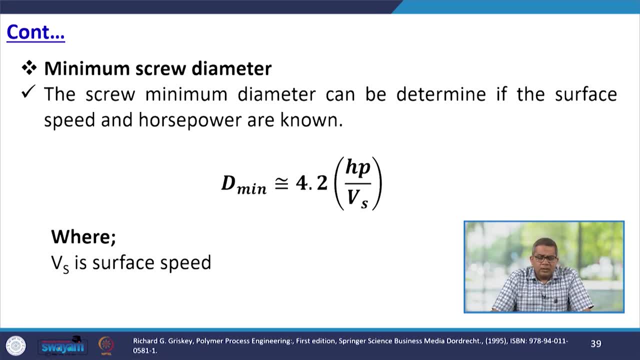 And TE and TF are the extrudate and the feed temperature. So E represents extrudate and F represents the heat temperature. The minimum screw diameter, the screw minimum diameter. this can be determined if surface speed and horse power are known. So this is the diameter. minimum diameter is equal to, almost equal to, 4.2 HP over VS. 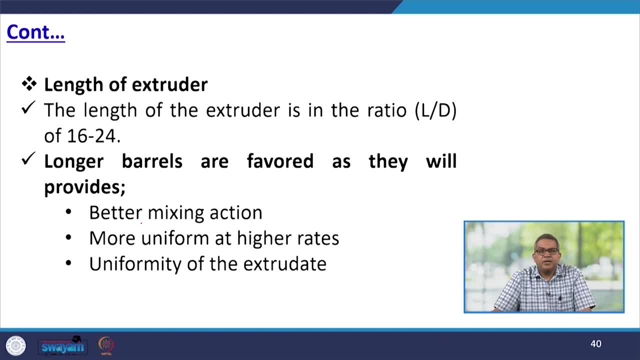 where VS is the surface speed. The length of extruder: again this is very important. The length of extruder is in the ratio L by D ratio of 16 to 24.. The longer barrels are favored as they will provide the better mixing action. 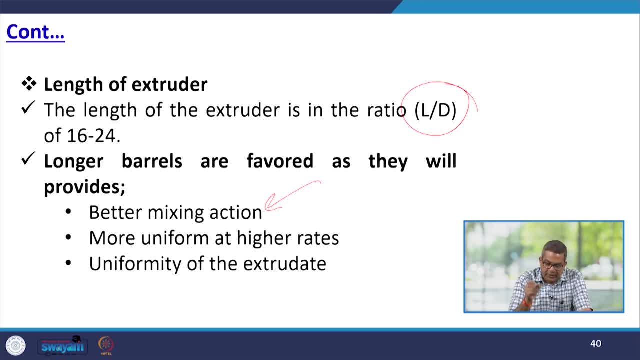 They will have a more uniform uh at high rates And uniformity of the extruder. The longer barrels are favored as they will provide the better mixing action. They will have a more uniform uh at high rates and uniformity of the extruder. 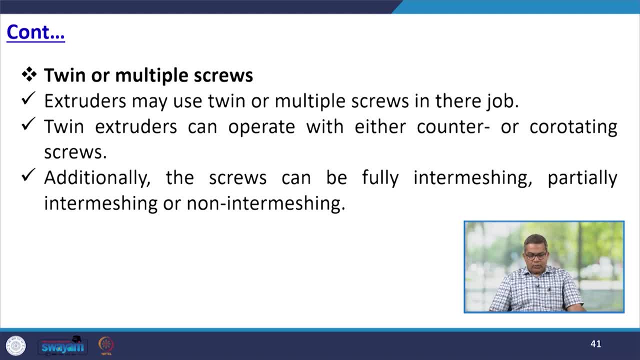 Vs is the surface speed. Now let us talk about the twin or multiple screws. The extruder may use twin or multiple screws in their jobs. Now, twin extruders can operate with either counter or co-rotating screws. Additionally, the screws can be fully intermeshing, partially intermeshing or non-intermeshing. 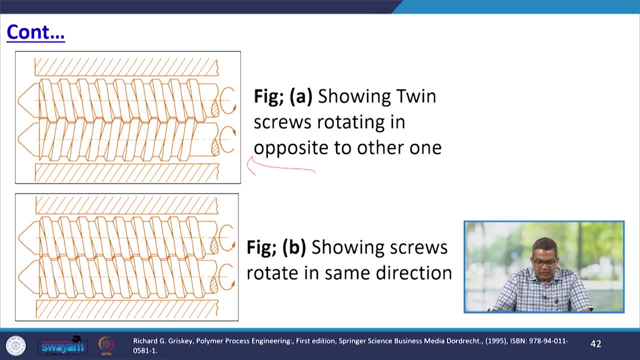 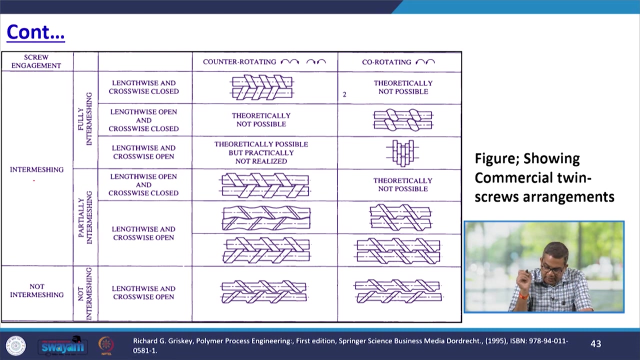 Now here you see, in this first figure, this showing the screws, the twin screws, rotating in opposite to each other. So it is like this: Here, in this particular figure, this reflects the screws rotated in the same direction. Now here you see that there are couple of things which we would like to have here, that 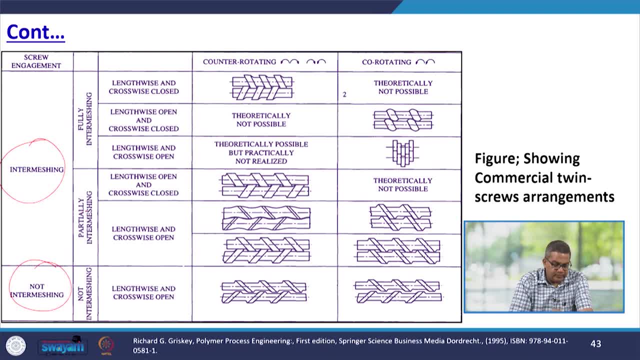 is screw engagement intermeshing and non-intermeshing. Now this is the two cases in intermeshing: the fully intermeshing and the partially intermeshing. Now the lengthwise, the fully intermeshing, they are subdivided into three aspects. 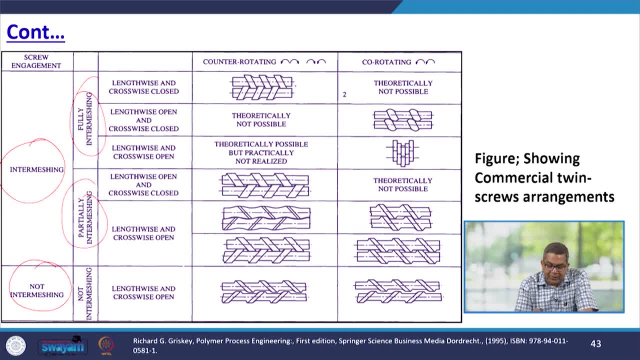 One is the lengthwise and the crosswise closed, like here. This is the counter-rotating and theoretically the co-rotating is not possible. Then the lengthwise open and the crosswise closed, which is not at all possible in the counter-rotating. 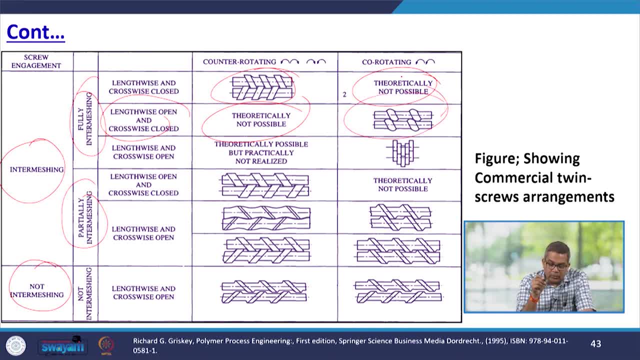 But it is possible in the co-rotating And the lengthwise and the crosswise open theoretically possible, but particularly when you are going for the economic aspect then it is not at all possible like this in the co-rotating. So when we discuss about the partially intermeshing the lengthwise open and the crosswise closed, 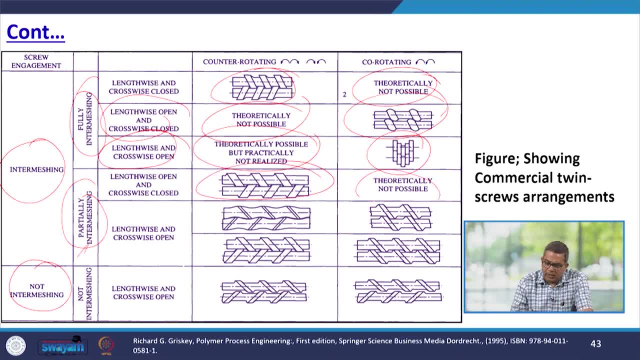 like this. You will see this in the counter-rotating and co-rotating is not possible. and the lengthwise and the crosswise open, You may have like this And in the co-rotating you may have like this type of the commercial twin screw arrangement. 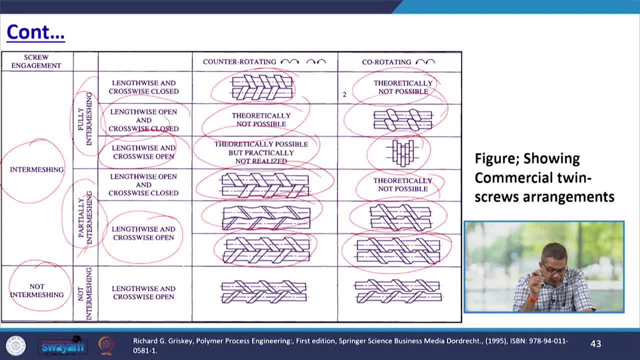 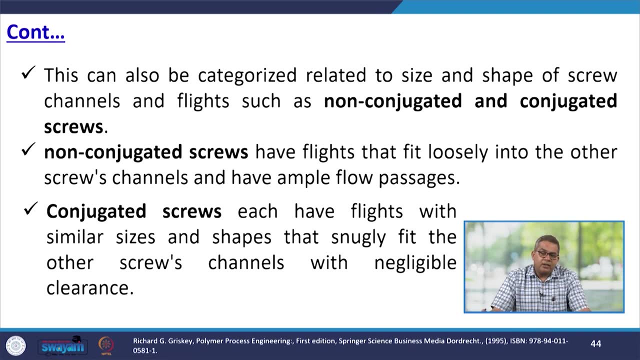 And when we talk about the non-intermeshing, the lengthwise and the crosswise open you may have in the counter-rotating like this and co-rotating like this, So this can be categorized related to the size, shape of the screw channel and the flight. 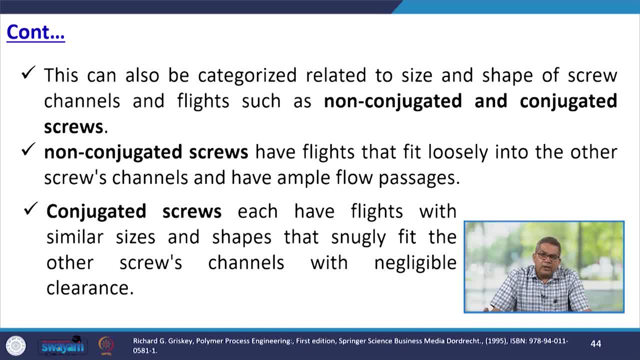 such as non-conjugated and conjugated screw. Non-conjugated screw have flights that fit loosely into the other screws channel and have ample flow passage so that there will be no locking etc. Now, conjugated screw each have the flights with the similar size and shape and snuggly. 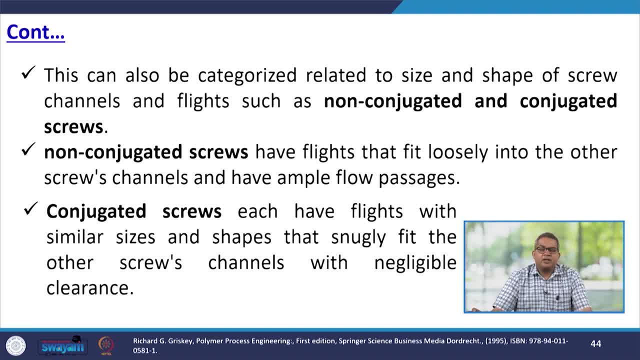 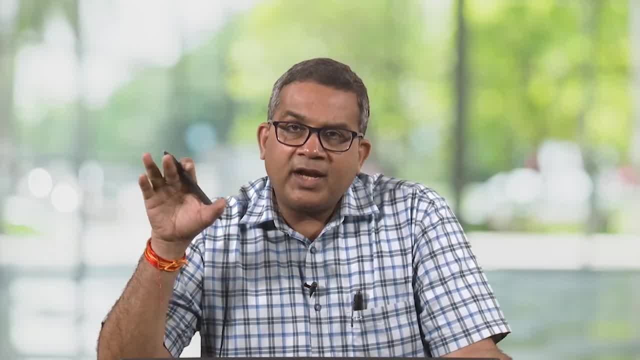 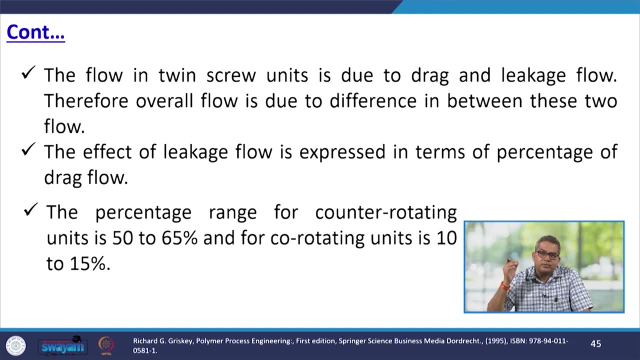 fit into other screws channel with the negligible clearance, so they will become more tight in nature. The flow in the twin screw unit is due to drag and leakage flow. Therefore, overall flow is due to the difference in between these two flows. The effect of leakage flow is expressed in terms of a percentage of drag flow. 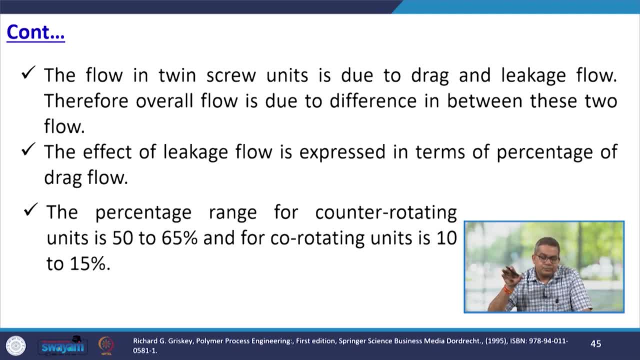 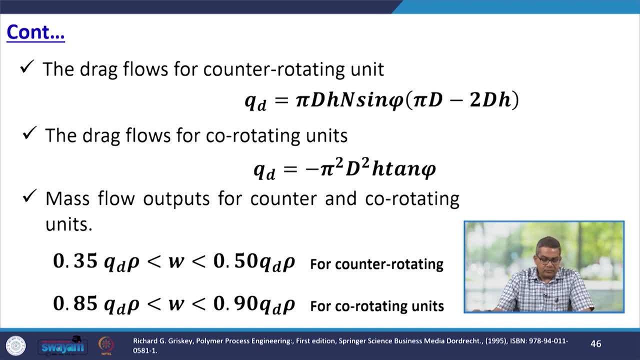 The percentage range from counter-rotating unit is 50 to 65 percent and for corotating unit is 10 to 15 percent. Now the drag flow for counter-rotating units can be categorized based on the co-rotation.